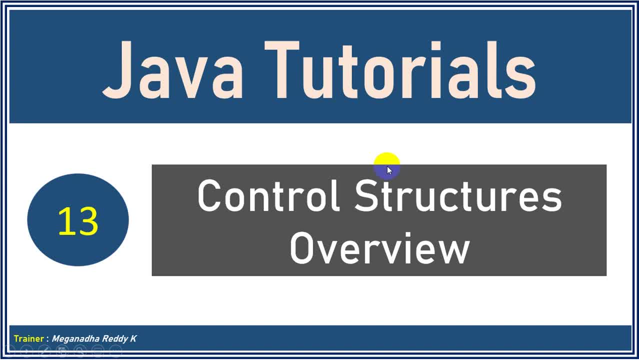 Hello everyone, this is Meghnath. Welcome back. So now we are entering into the next phase of programming of Java tutorials: control structures. So far, we learned about how to write simple hello world program data types and we learned about operators and we learned about operator. 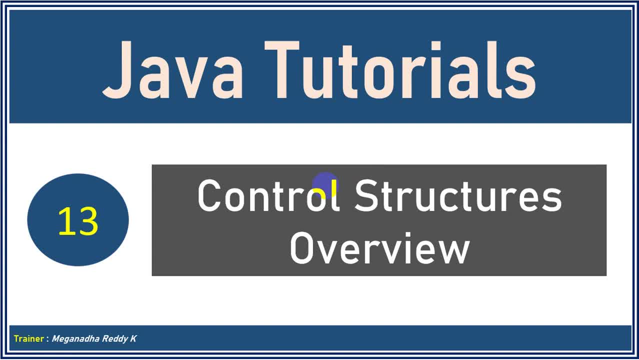 precedence. So all those things will form your foundation and from now, whatever we're going to learn will give you some real good idea about how we have to write some programs, how to write some business logic. So from here, it's all important that you should keep practicing in Eclipse IDE. 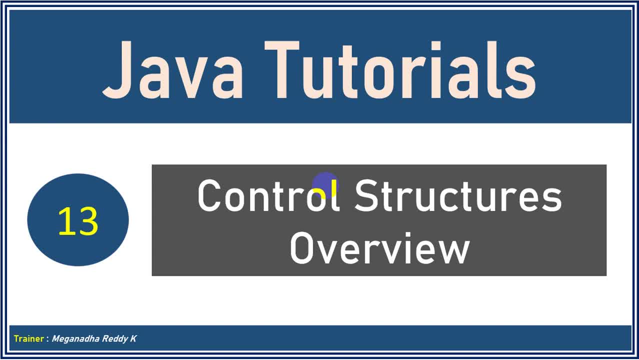 and see how the output works. So now in this module we talk about control structures, a high level overview From the next module we talk about in depth, about each control structure, and you have to practice it from the next lecture. So make sure that you have Eclipse IDE installed and keep. 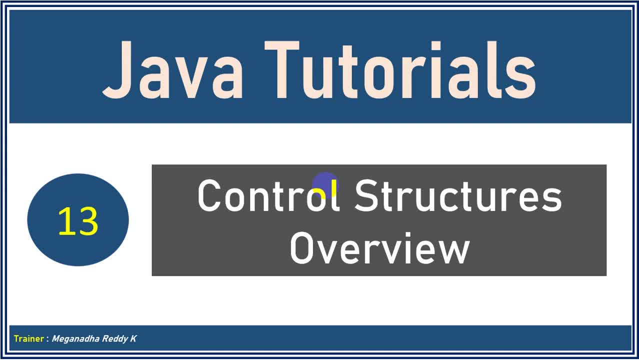 practicing from the next module, right? So with that, let's get started. Now, when you're writing some program, you need to take some decisions. Let's take you're working on something like a retail retail project Where if a person buys 3 quantity, you have to give 30% discount. and let's take, if a 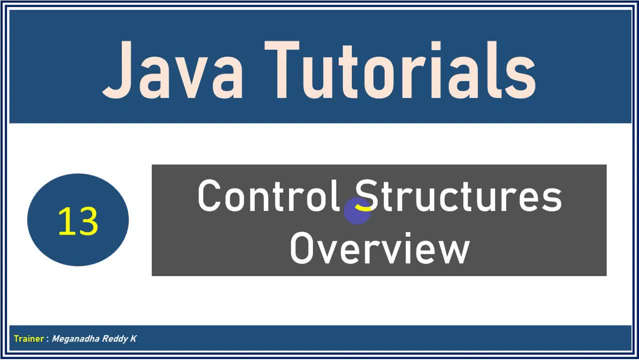 person buys quantity as 4, you have to give 40 percent discount. So in this case, based on the quantity that customer has purchased, you have to take some decisions, So you have to. your code control flow should travel either: based on the discount should be 30 if it is quantity 3, if it is 4. 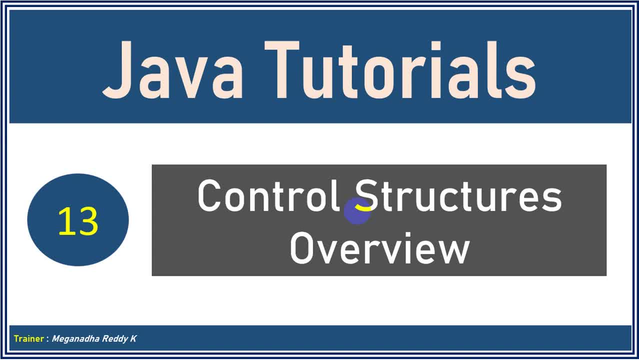 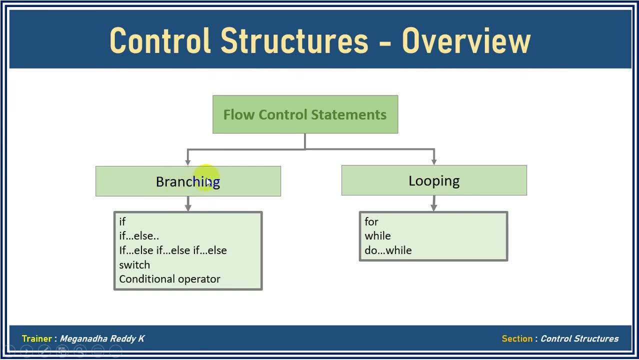 the discount is 40 percent. so you have to take the control and you have to decide which logic you have to write, so so that logic deciding factors and decision making steps comes under control structures. now, control structures are categorized into two types. one is branching where you want to. 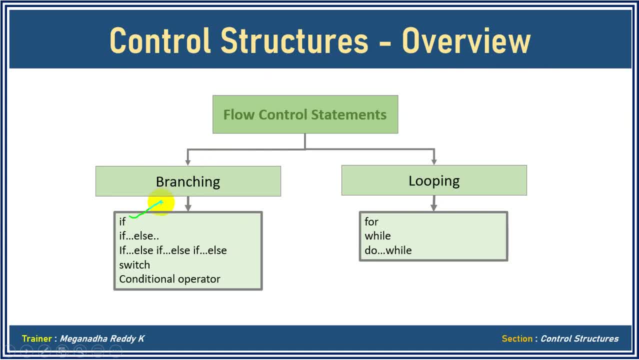 take a decision based on something. if this is, if this quantity is four, give the discount as 40 percent. so if the discount is three, give. so if decision making comes under branching, if there are multiple options, like if the person buys two, give some discount, if the person buys three, give. 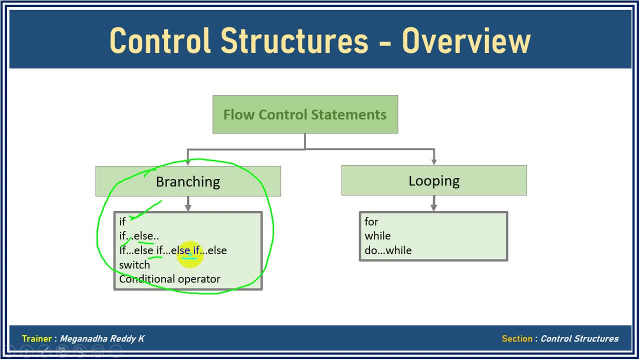 some discount. the person buys four, give some discount. if something above five, give something discount like this. so in switch case, if you have multiple options and then get better to go to switch case, we're going to see that as well in in detail in the further modules and also we talk. 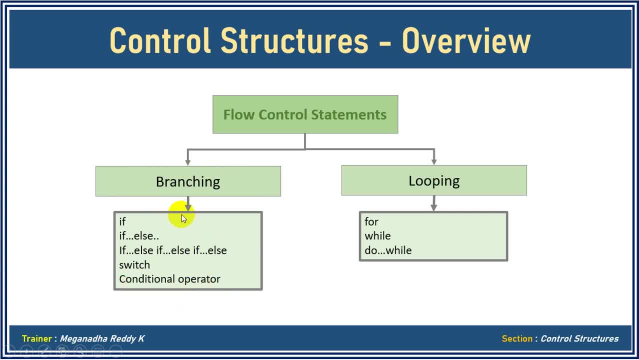 about conditional operators. so all these modules or all these topics that i mentioned here comes under branching, because when the code flow is happening, based on the condition, you select one option. again based on the condition, you select one option. so this looks like branches of a tree. that's why these are. 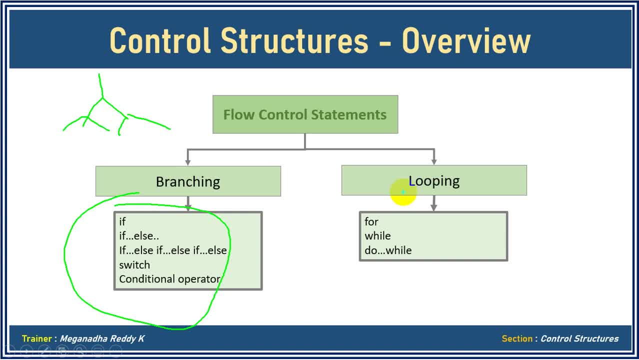 called branching. now looping means iterating same task multiple times. so for loop, let's take i want to print hello five times, or while loop, same, where you need, you need to loop. so again, some people are here calling if as a loop. so if someone says like if loop and is wrong, if is not a 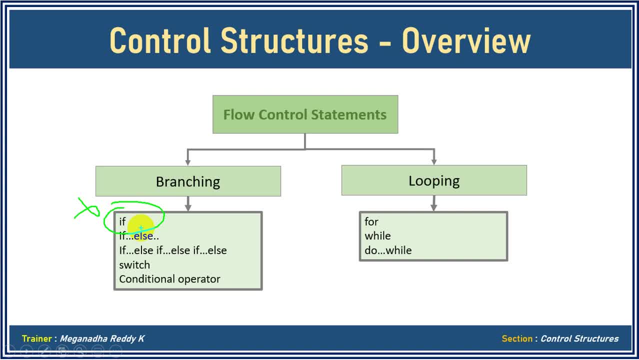 loop if is just a condition. if the condition is satisfied it will just print the statements inside it. otherwise it'll skip the statements inside it. so if is not a loop, so never speak like use if loop, there you have to use if condition when you're saying: for you can use definitely loop, it'll. 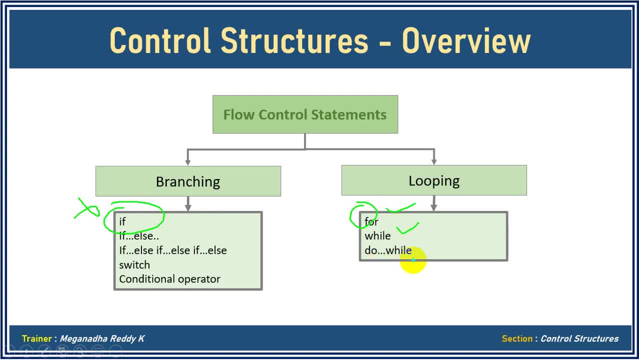 iterate multiple times. while we'll iterate multiple times, do while we'll iterate multiple times. so these are called looping concepts. so so conditional or control structures are two types. one is branching and looping, and we'll talk about more this branching and looping in detail in the further. 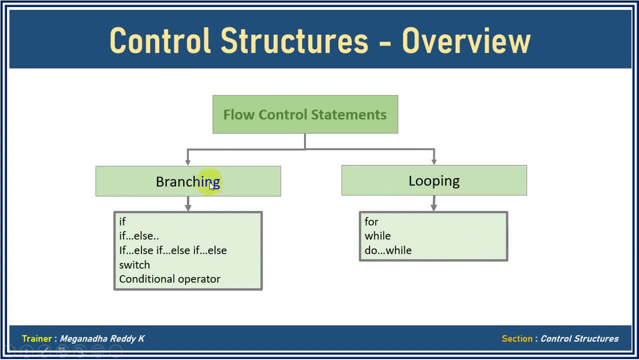 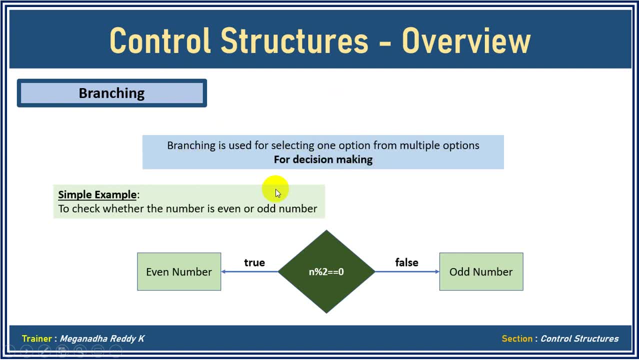 modules. so let's see what is branching in a very high level. so branching branching is used to select one option from multiple options for decision making. for example, a simple example: i want to check whether the given number is even or odd number, so i'll write here if n modulo 2. 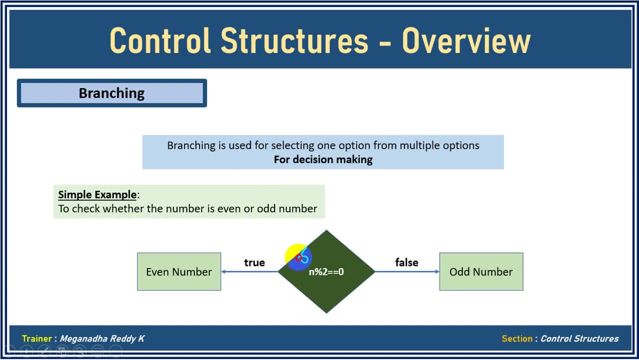 so modulo 2 is used, to see the reminder. so if let's take, there is number 6. if 6 modulo 2- and i use to check equal to or not using double equals to- is 0, now obviously 6 modulo 2 is 0 if it is. 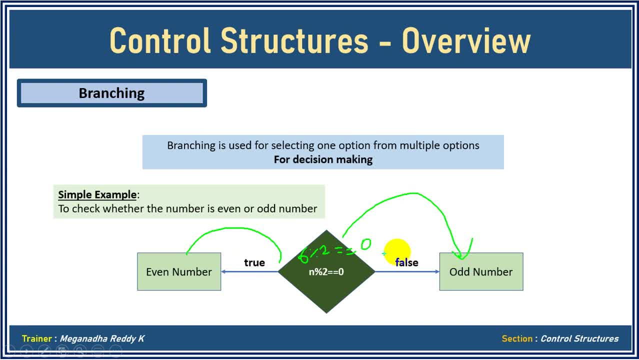 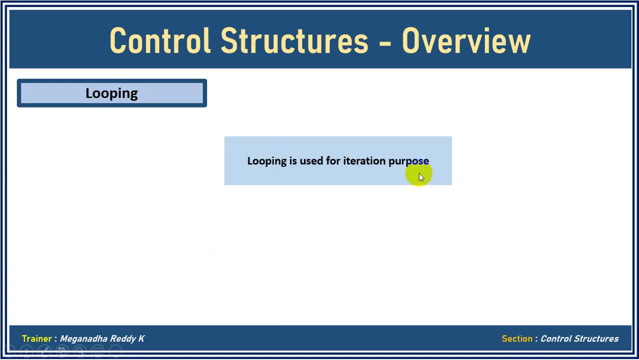 satisfied, i'll print even number. else i'll print odd numbers. so this is called branching, so only one. we are doing it in this. now we talk about what is looping. now looping is used for iteration purpose. a simple example could be: i want to print hello five times. 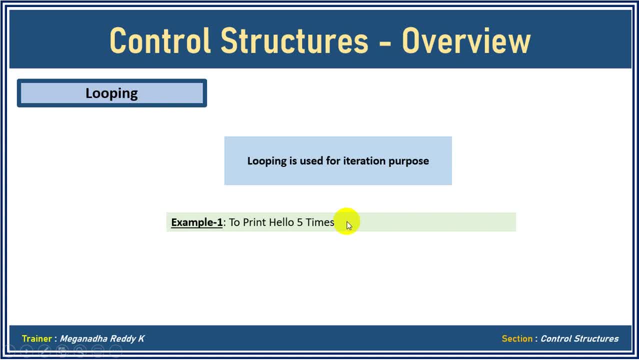 where i'll write a for loop from one to five and print hello, hello, hello and it'll. it'll actually print five times. we're going to see examples when you talk about for loop in detail in further modules. and second example could be: i want to find sum of n natural numbers, so i'll write a loop from: 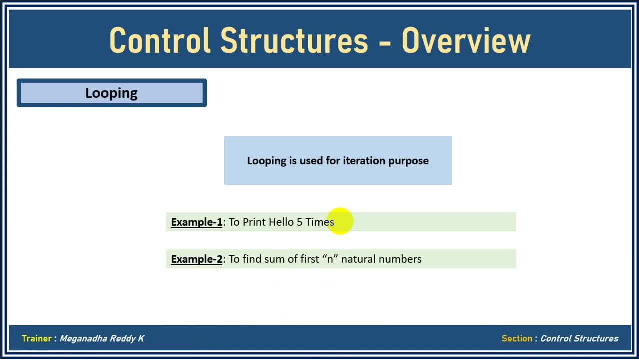 one to n and i keep on adding that number to the sum. so to find the sum of n natural numbers. so here we are iterating, we are adding some n times, one plus two plus three, plus four, up to n times. so we are using a loop here and similarly to check whether the number is even or odd number. so i'll 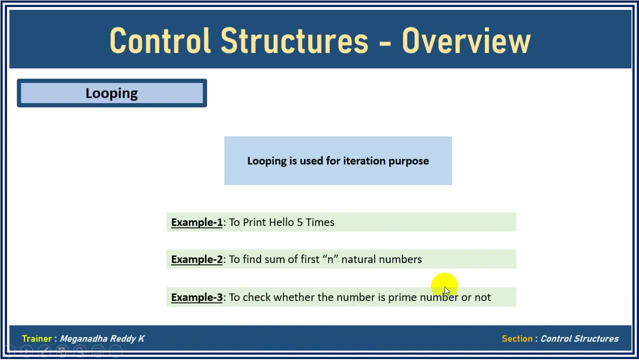 write a loop here and similarly to check whether the number is prime or not. so you have to divide the given number from one to n, keep checking whether the number is digital by one, two, three, four, like that. so again, this is also iterative purpose. so these are some of the examples where 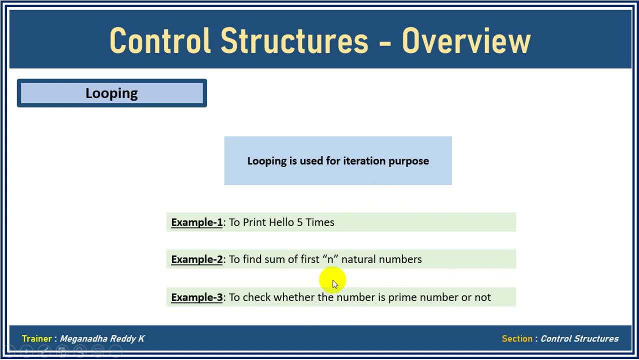 we will use looping. so branching is a decision making, looping is iterative purpose and in the next modules we talk about in detail about each one in branching and looping. so i hope you got some clear idea about control structures. what is branching and what is looping and what? 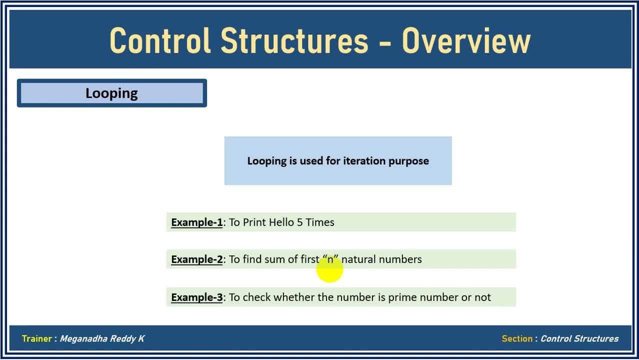 we have inside branching like if, if else, else, if else, if else, if and all, and we have a switch case and we have conditional operator and in in looping we have for loop, while loop and do while loop. so we're going to discuss in detail in further modules. so thank you and see you in the next module. 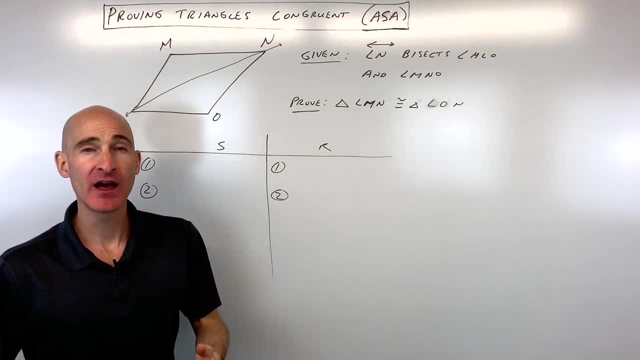 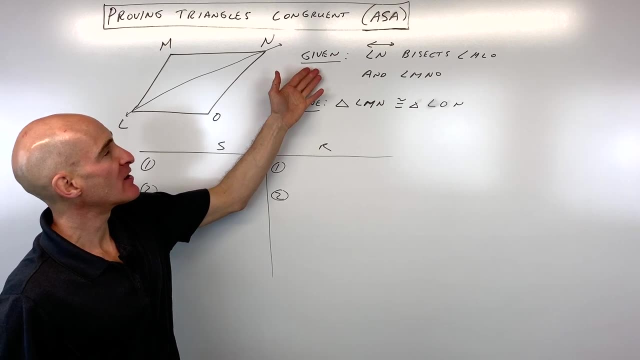 Triangles congruent. I'm going to show you a process that I use and I help students kind of work through so they don't get stuck when they're doing these two column proofs. The first thing I like to do is kind of just look through the problem and kind of see what I can figure out. 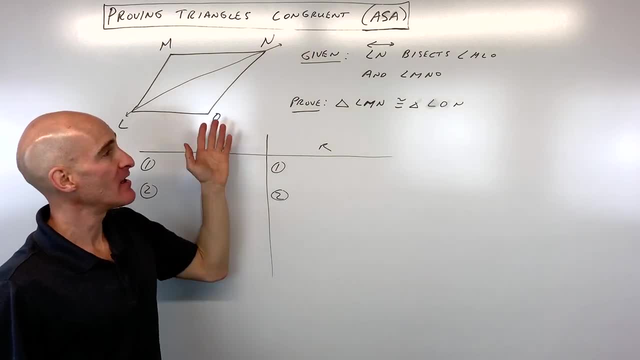 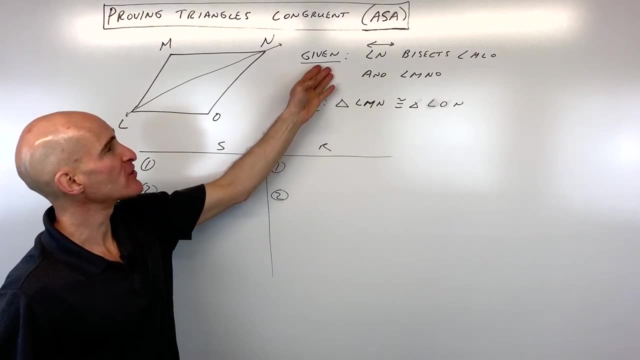 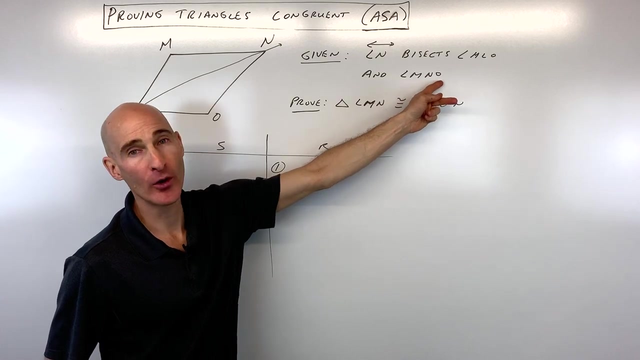 from the givens first, then from the diagram second, then, if I have to, from previous steps. you know you can figure out some additional quantities that are congruent. So the first thing I do is take the givens, I say okay, line LN bisects, angle MLO and angle MNO: Okay, 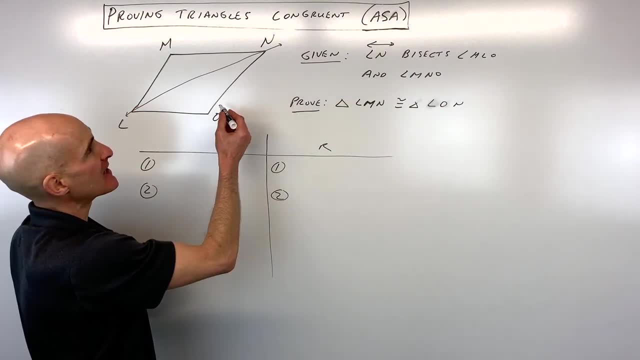 so let's look at that. So here's line LN. It's bisecting angle MLO, So it means it's cutting it in half. Bi means two, sect means cut, So it means that these two angles are congruent. So I 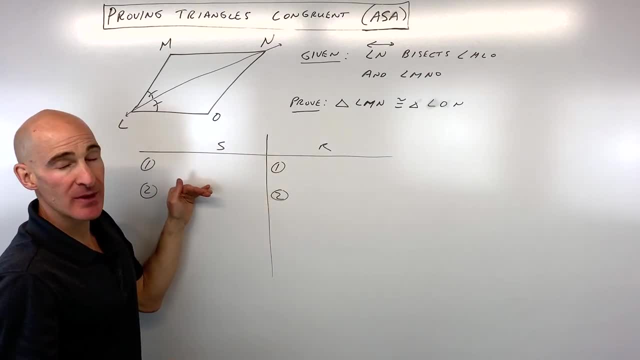 like to mark it on the diagram, And then, when I figure things out, I also like to make it a step in my proof. So I'm going to go ahead and put that down. Let's see it's angle. MLO, Whoops.